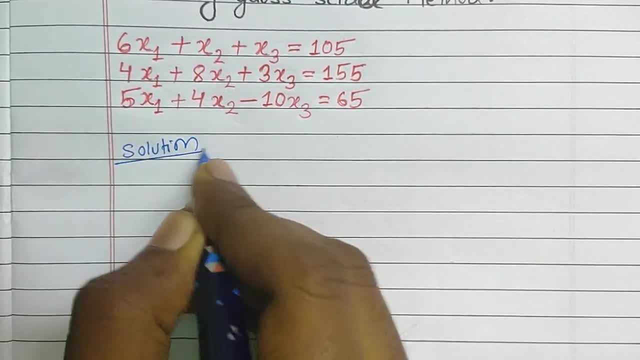 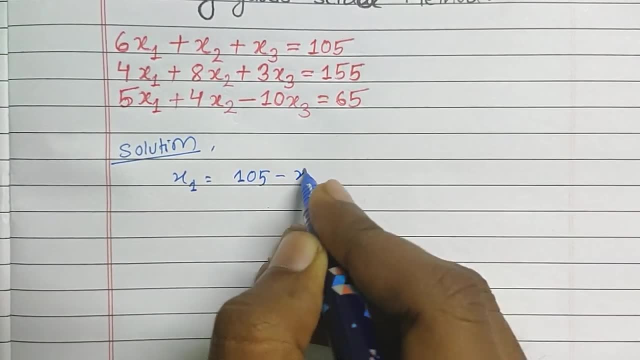 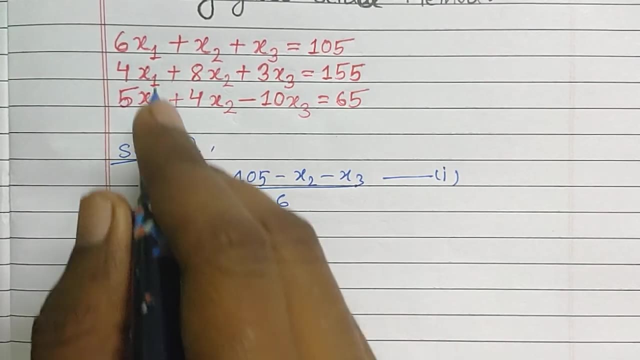 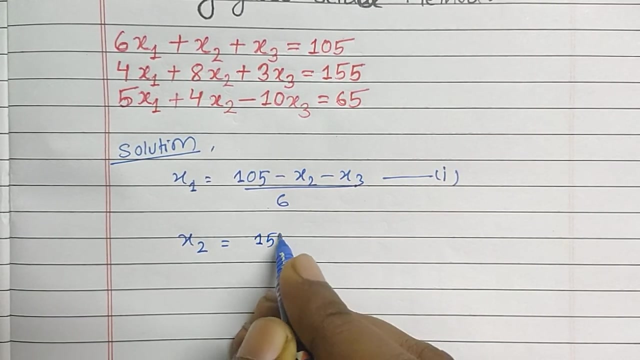 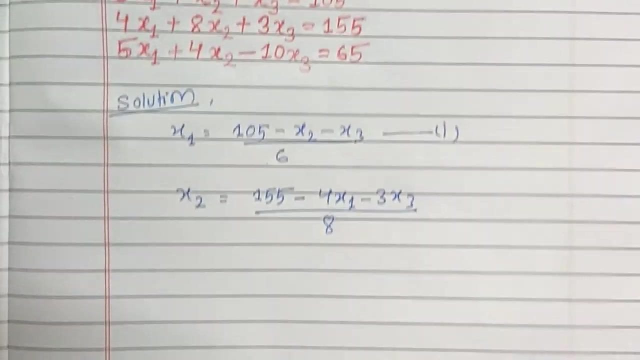 the solution is from equation 1. what we will have is: x1 is equal to 105 minus x2 minus x3 by 6. this will be our equation 1. again from second equation, we will have: x2 equals to 155 minus 4, X 1 minus 3 X 3 upon 8. this is our equation 2nd. 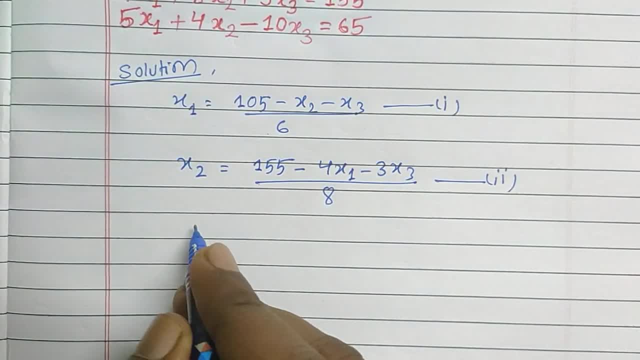 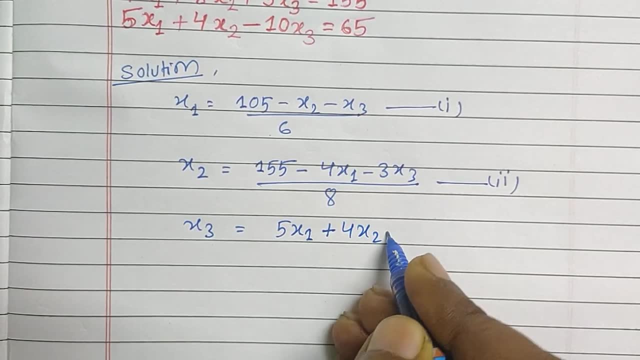 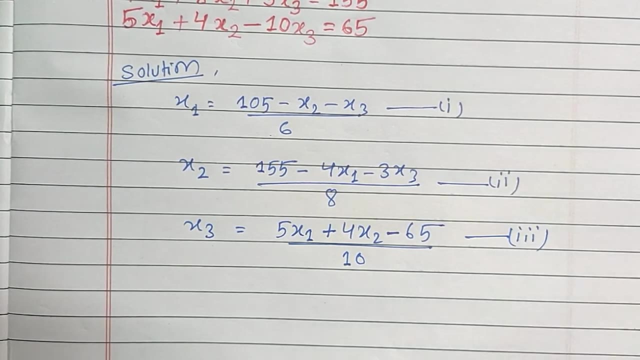 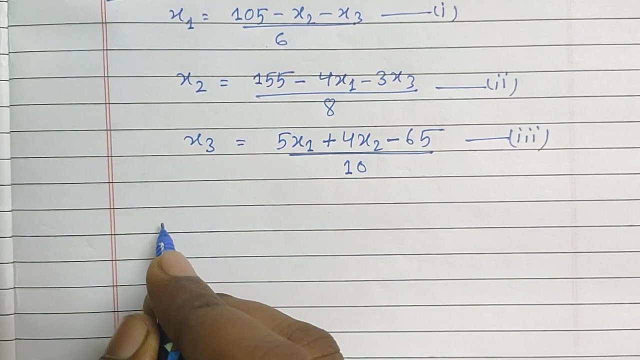 again from this third equation we will have: x3 is equal to 5 X 3 대박 x1 plus 4, x2 minus 65 upon 10. this is our equation. third now, while moving on with the solution, we have to move on. taking x2 is equal to 0 and x3 is equal. 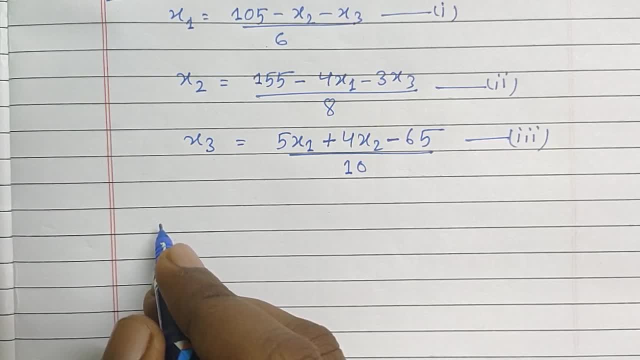 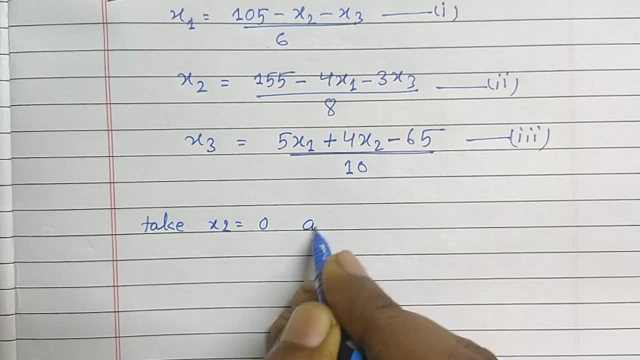 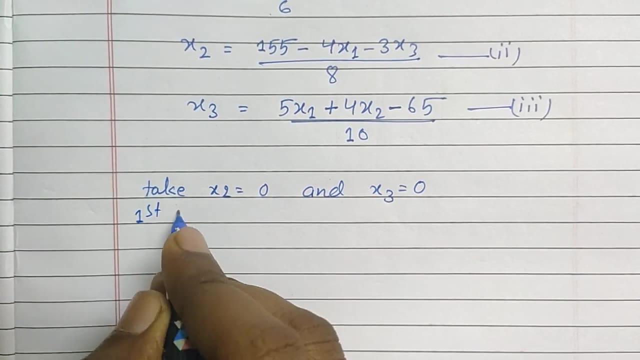 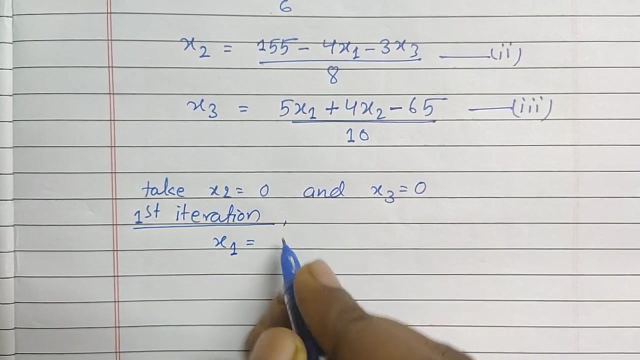 to 0, so that we would be able to find the value of x1 in first iteration. so take: x2 is equal to 0 and x3 is equal to 0. now for first iteration iteration, what we will have: x1 is equal to 105 minus 0. we have to put the value of. 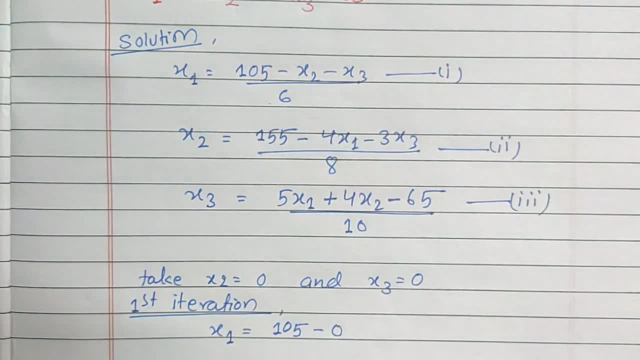 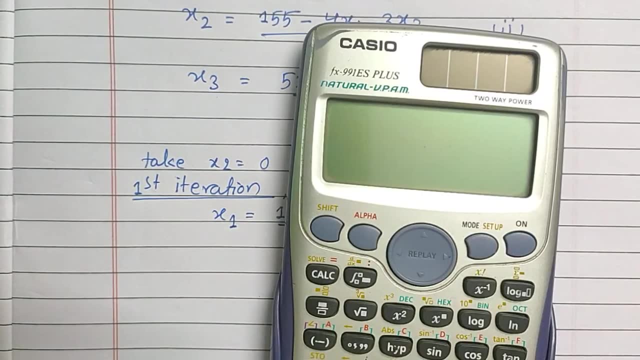 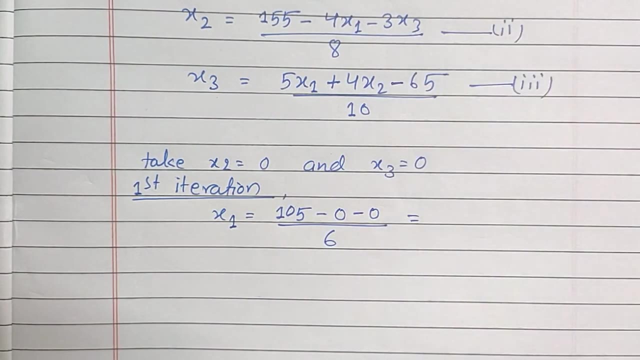 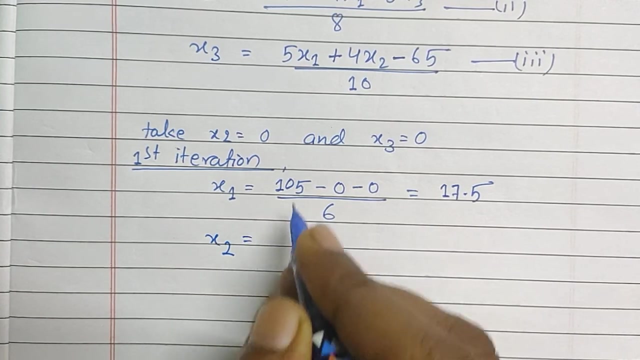 x2 is equal to 0 and x3 is equal to 0 in first iteration. So this will be 0 minus 0 upon 6 and we will have 105 divided by 6.. This is 17.5.. Now for x2, we have the equation 155 minus 4x1 minus 3x3 upon 8.. 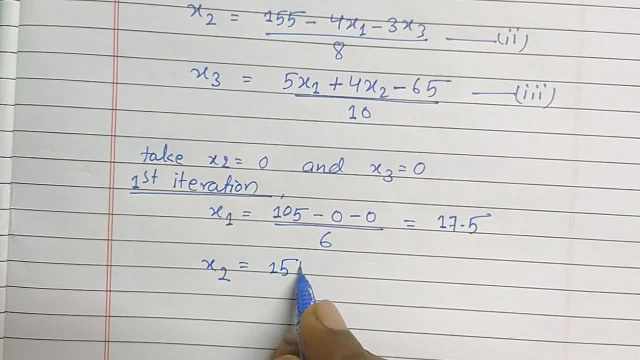 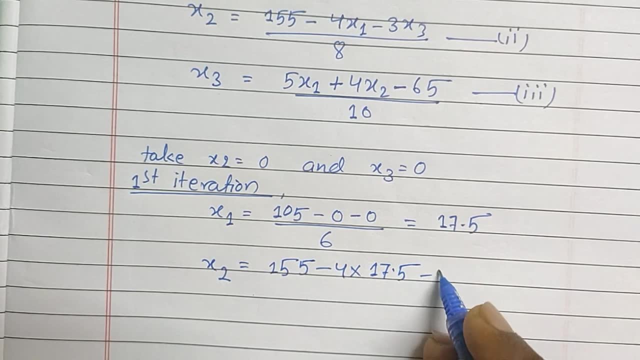 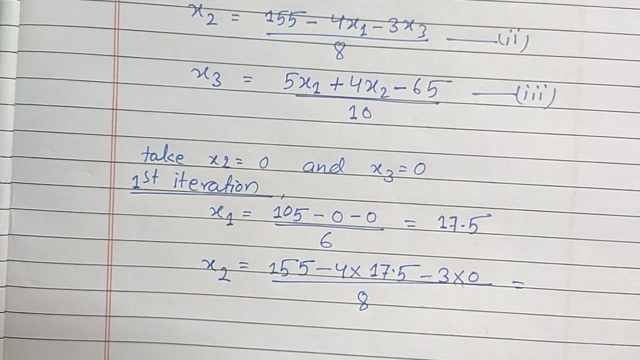 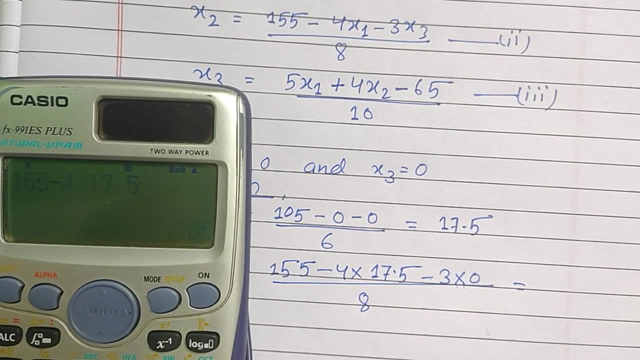 So this will be 155 minus 4 into x1, will be this value: 17.5 minus 3 into x3 is 0.. So put it here and divide by 8.. You will get the answer from here, which will be 155 minus 4 into 17.5 divided by 8.. 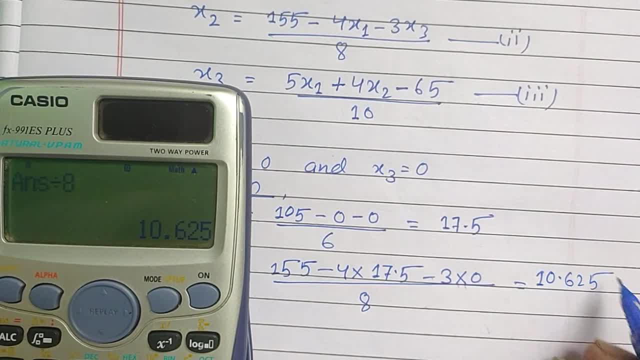 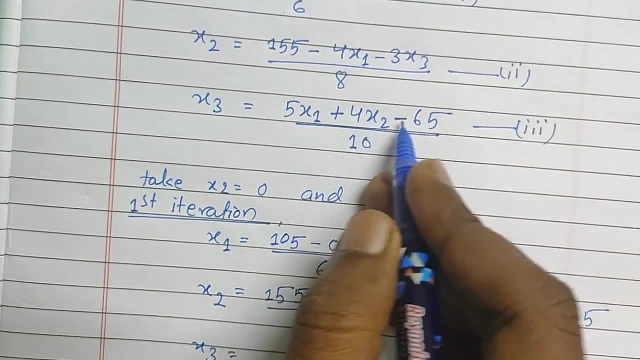 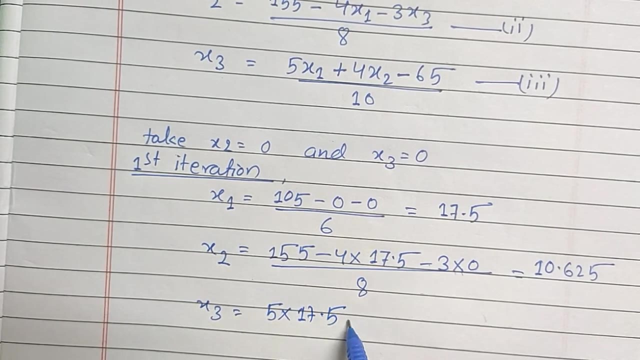 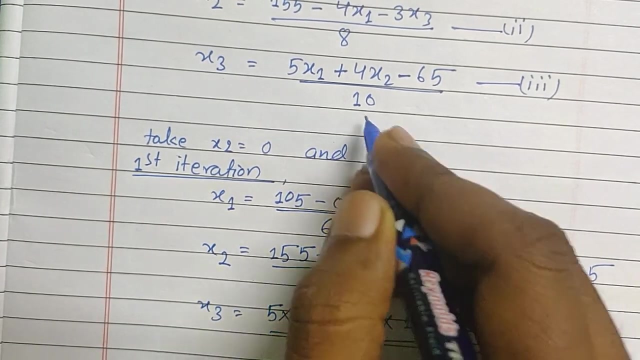 This is 10.625.. Now the time for x3 equation is 5x1 plus 4x2 minus 65.. So put the value 5 into x1 value is 17.5 plus 4 into x2 will be 10.625 minus 65 divided by 10.. 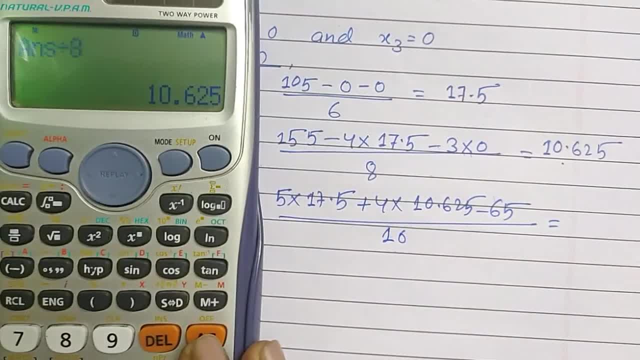 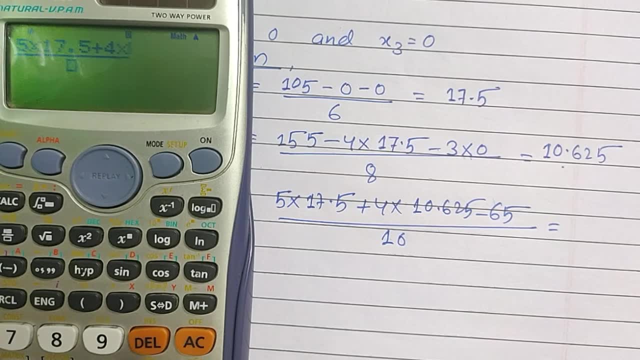 Now solve this using calculator and you will get the answer of x3, which will be 5.. 5 into 17.5.. 5 into 17.5, plus 4 into 10.625, minus 65 divided by 10.. 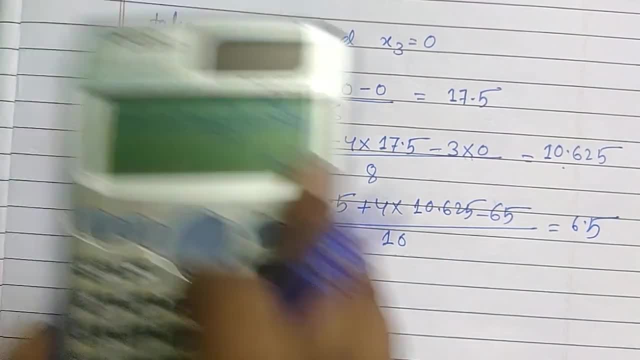 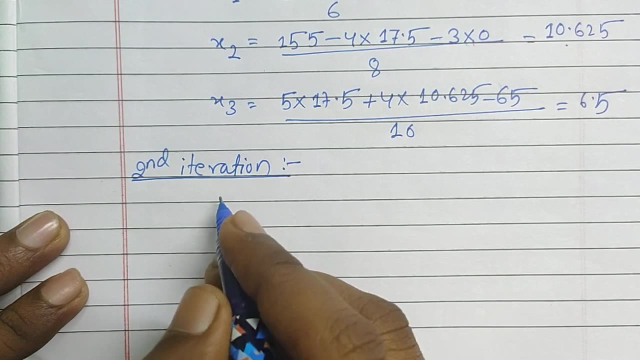 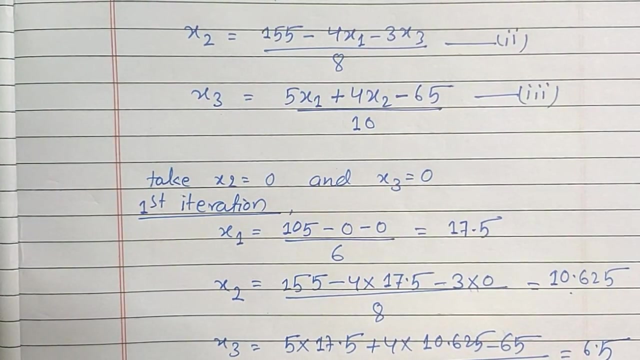 The answer is 6.59.. Now let's move for the second iteration. Now for second iteration. what we need to do is we again need to find the value of x1.. And equation will be the same: 105.. 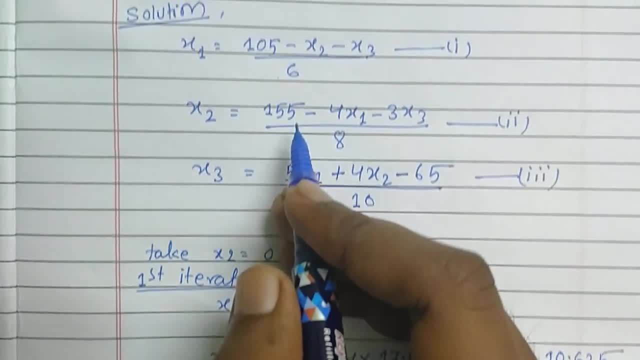 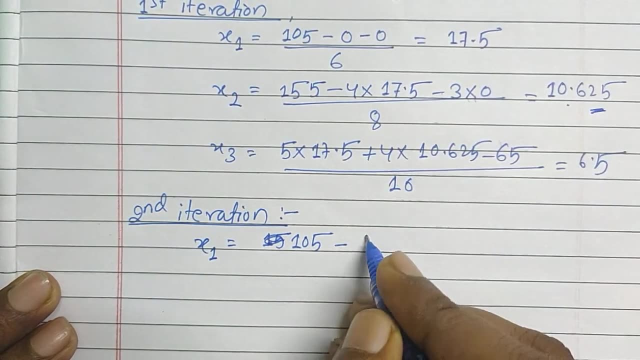 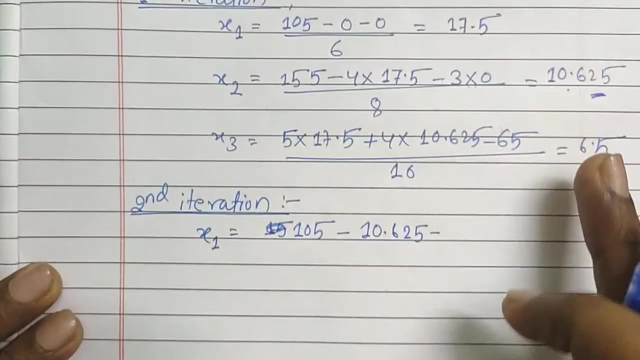 105.. Minus Here, the equation is 105 minus x2.. And here the value will be this: 17.625.. 10.625 minus here, x3.. So the x3 will be 6.5.. 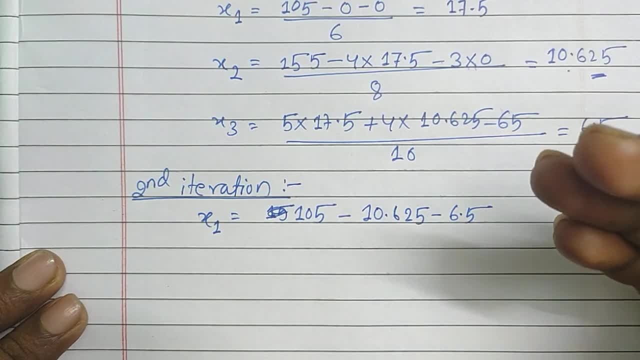 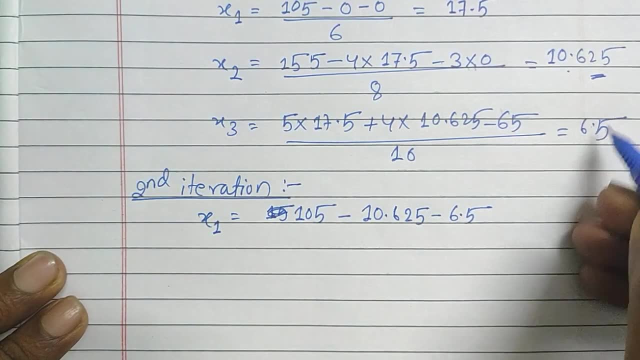 We have to take the value of the preceding iteration. So here the preceding iteration of second iteration is first iteration. So value of x2.. And x3 will be 10.625 and 6.5 respectively. Now put the value. 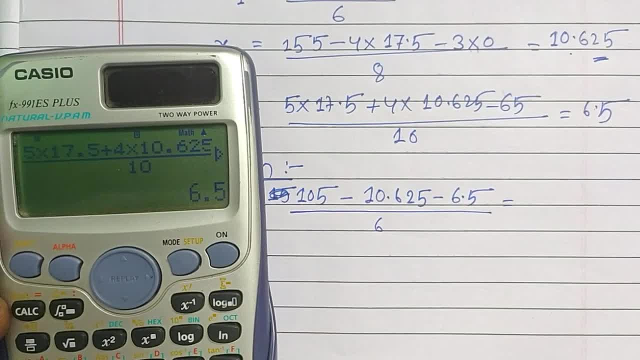 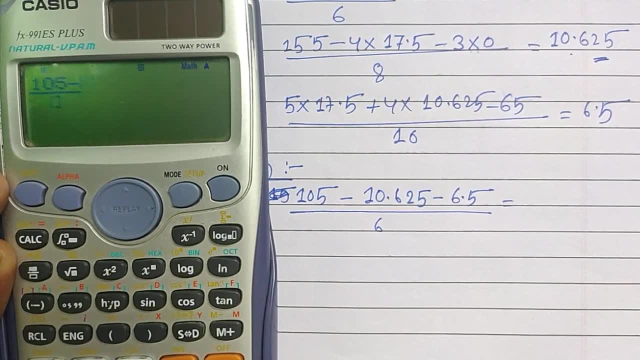 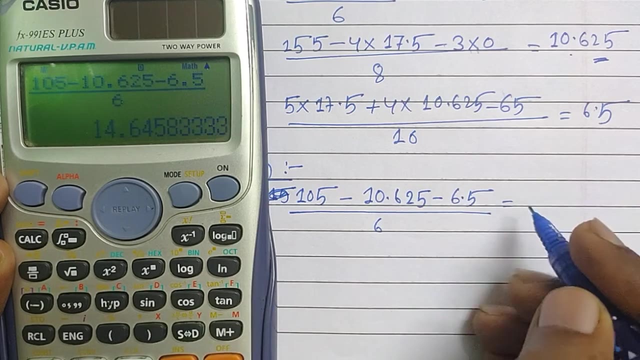 And you will get the value of x1.. Here the value of x1 will be 105.. 105 minus 10.625 minus 6.5, divided by 6. The answer will be 14.645.. Now time for x2.. 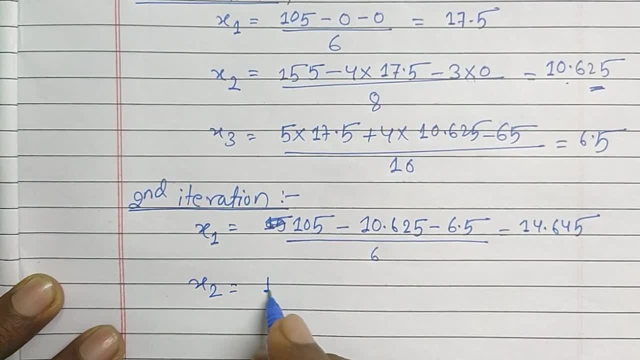 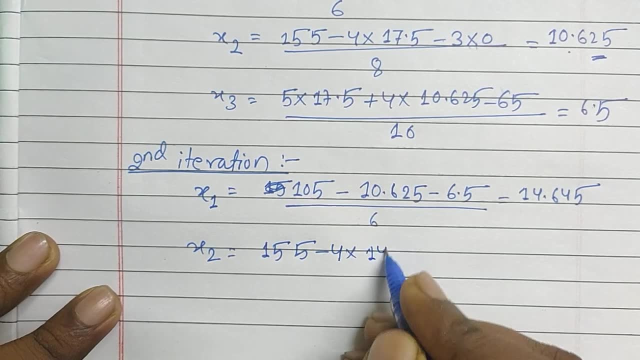 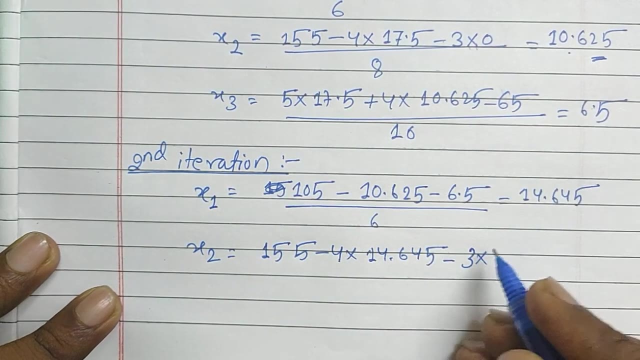 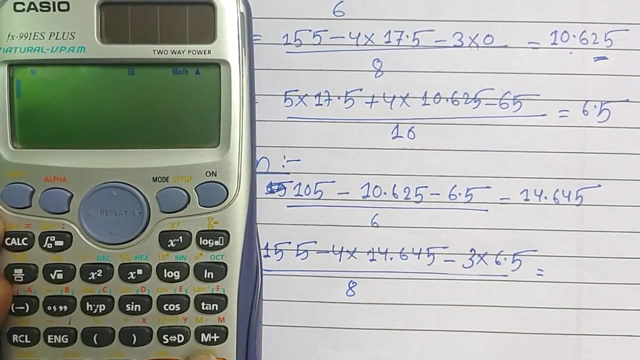 So the equation is 155 minus 4 into x1. And x1 value will be 14.645 minus 3 into x3. And x3 will be this value, 6.5 upon 8. You will get the answer, which will be 155.. 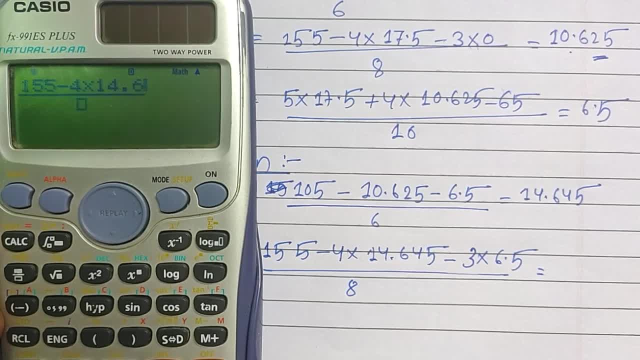 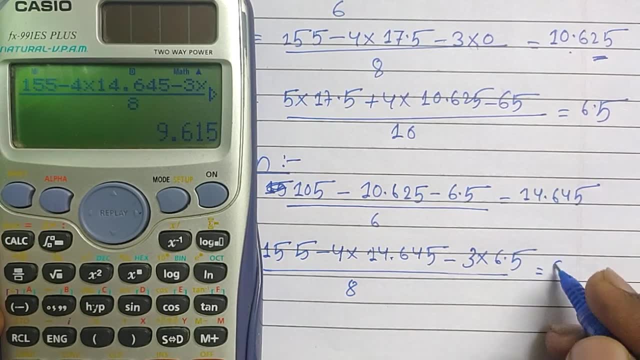 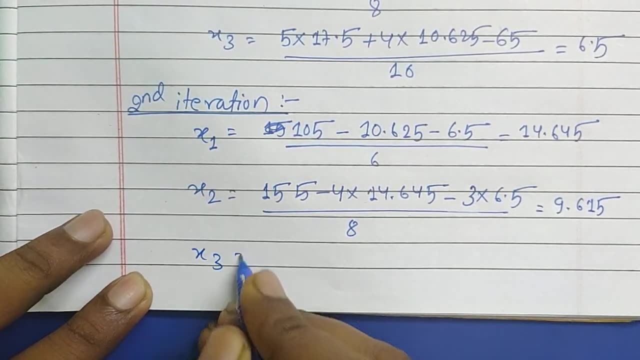 155 minus 4 into 14.645, minus 3 into 6.5 divided by 8.. So the answer is 9.615.. Now find the value of x3.. x3.. The equation is 5 into x1.. 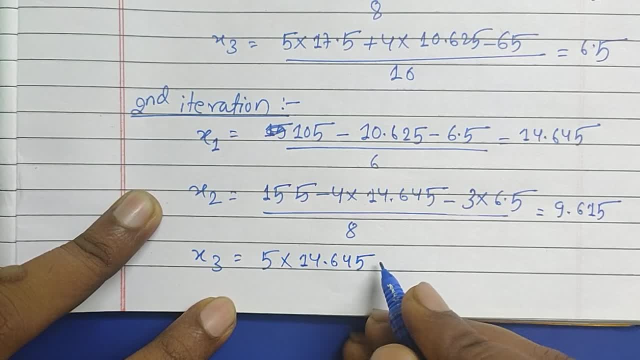 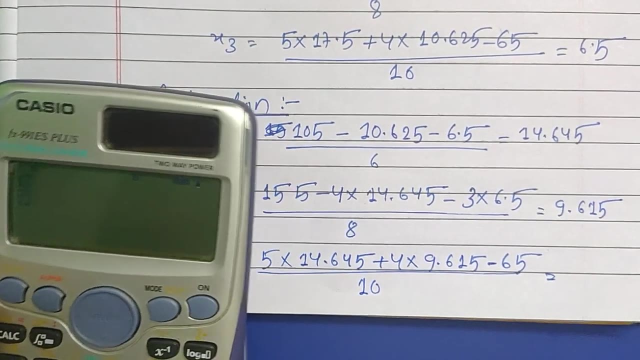 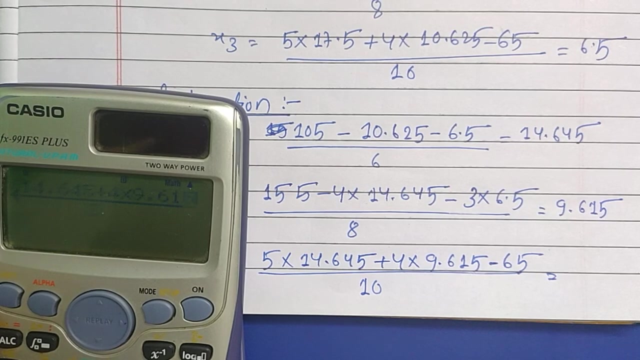 So 14.645 plus 4 into x2 means 9.615 minus 6.5.. You will get the value of x2.. Now the equation is 155.. So 155.. So x2 is 9.615.. 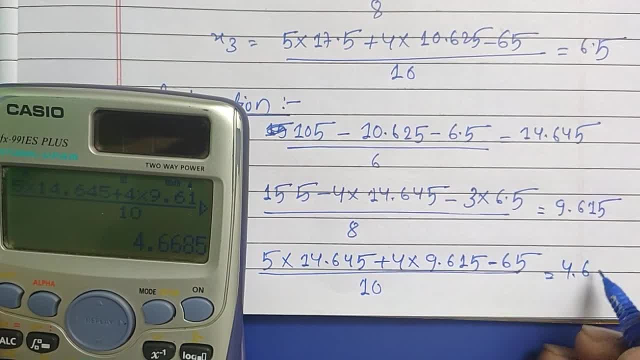 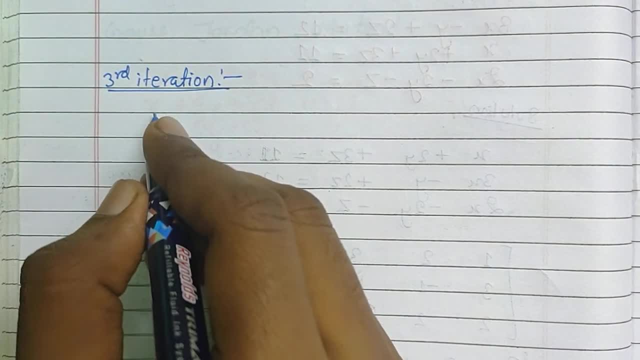 Were you ask for that, So x2.. So x2 equals 16.661 over 16.615.. Once again, you will get the question in the next minutes And and then you will swing it, So x2, which is 9.615.. 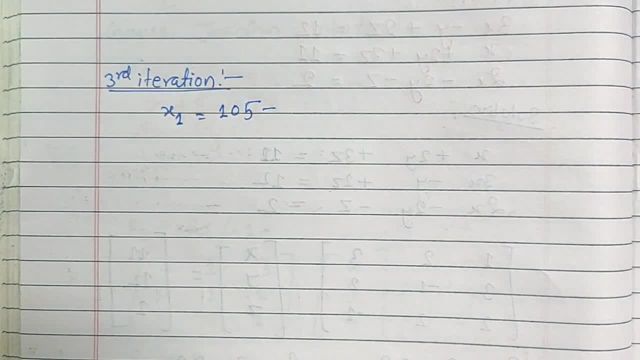 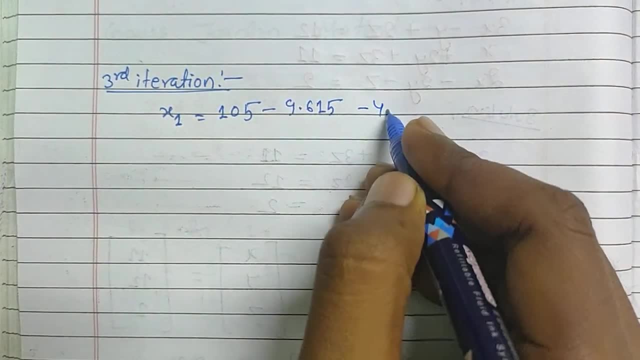 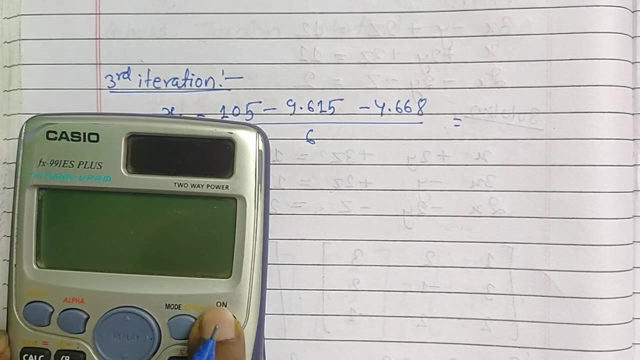 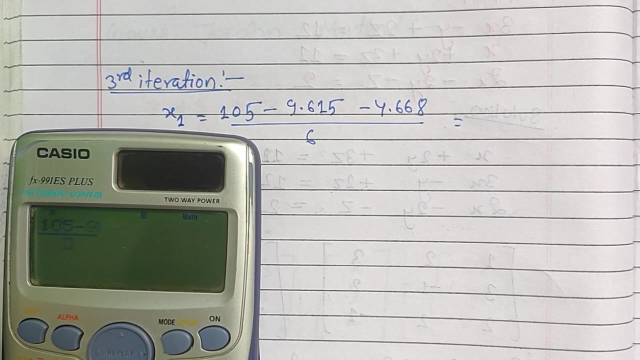 is equal to 105 minus x2. the previous value of x2 was nine point six one five minus x3. x3 was four point six six eight divided by six. let's check the answer. what will get? the answer is 105 minus nine point six one five minus four point. 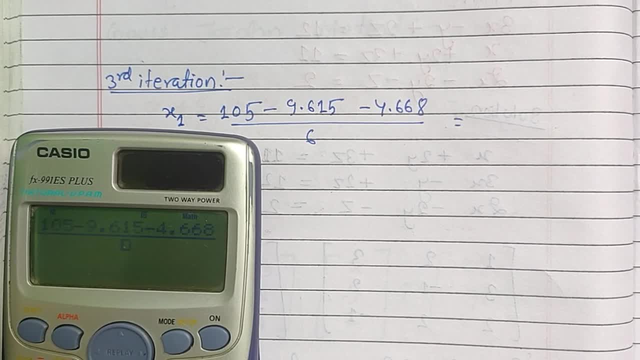 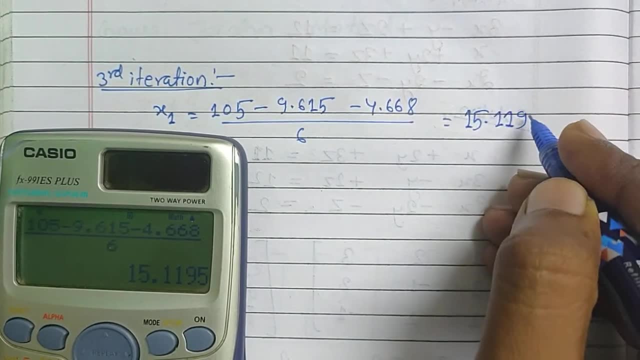 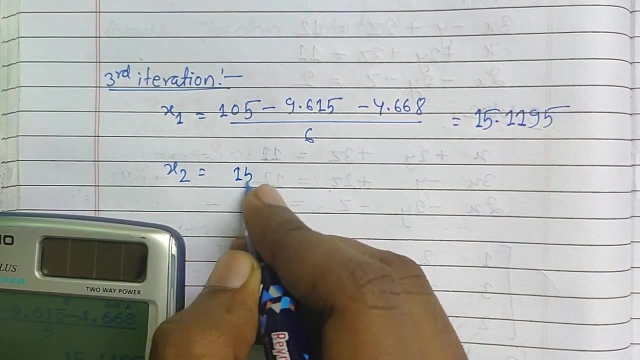 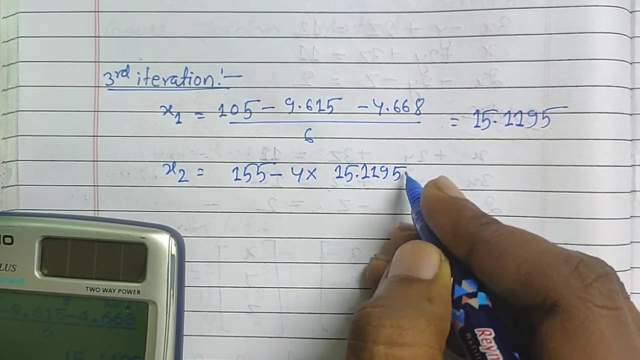 six, six eight divided by six, and the answer is fifteen point one, one nine five. again x2 will be x2 will be one hundred fifty five minus four into X one will be fifteen point one. one nine five minus three into x3 is four point six. 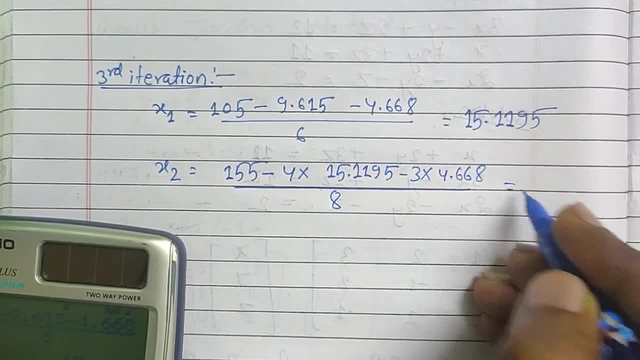 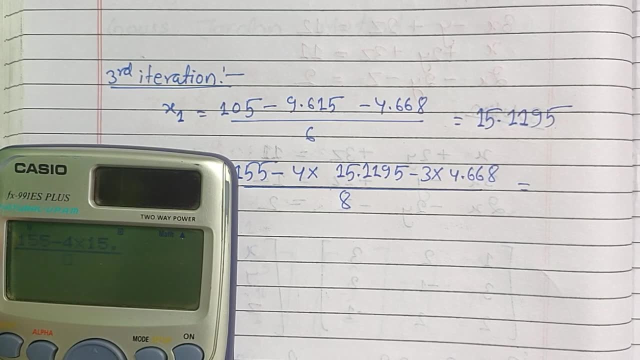 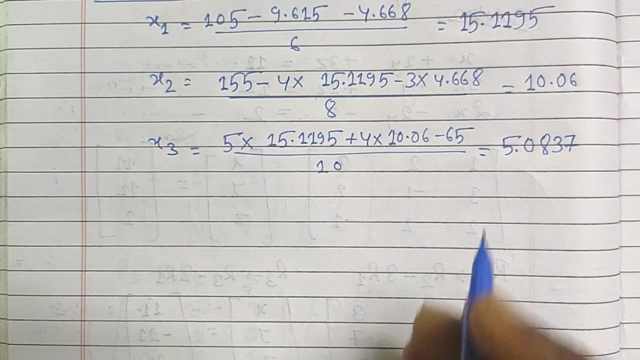 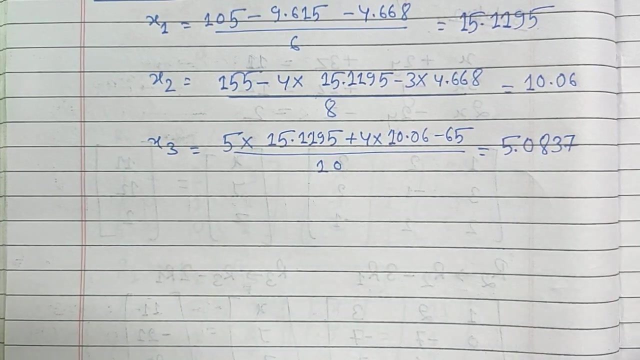 six eight Divide by 8.. The answer is 155 minus 4 into 15.1195, minus 3 into 4.668.. Divide by 8. The answer is 10.06.. Here the value of X3 will be 5.0837, on putting the value of X1 and X2 in the, 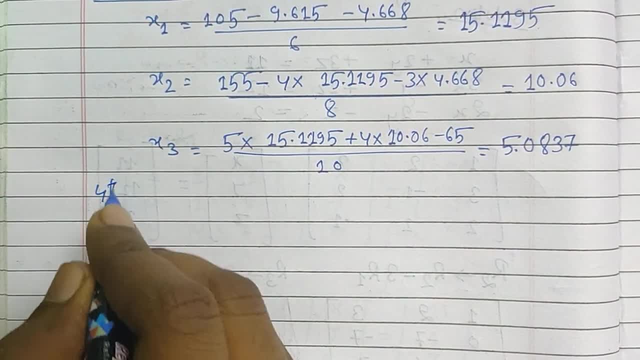 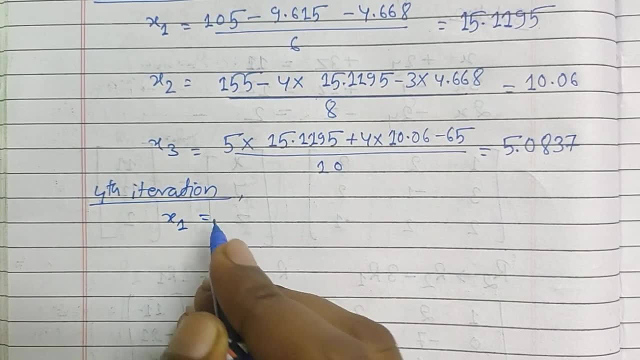 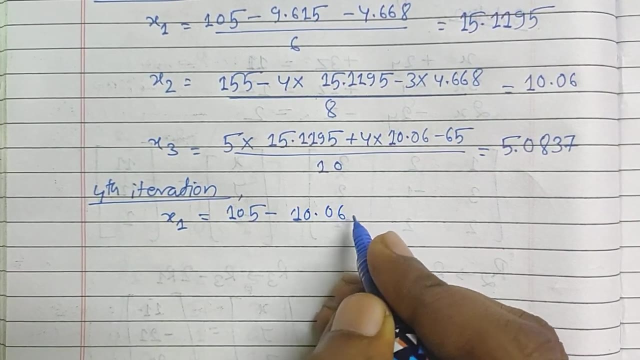 equation 3rd. Now let's move toward the 4th iteration. Again, in 4th iteration we need to find X1,. for X1, the equation is 105 minus X2.. X2 will be 10.06 minus X3,. 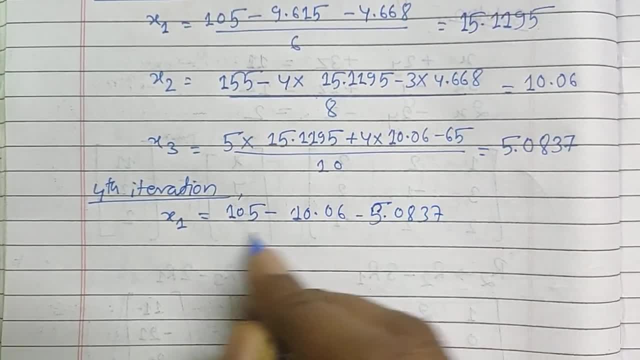 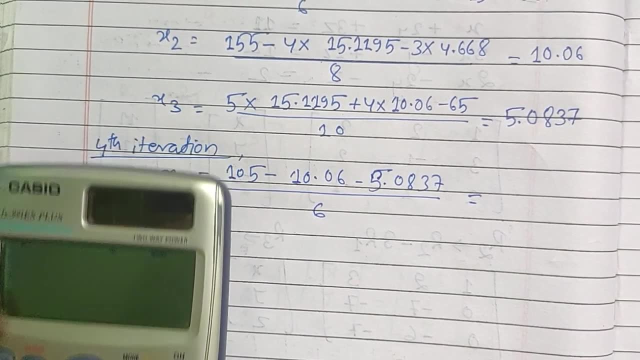 X3 is 10.06 minus X3.. X3 will be 10.06 minus X3.. X3 is 10.06 minus X3.. X3 is five point zero, eight, three, seven. divided by six, the answer will be 105. 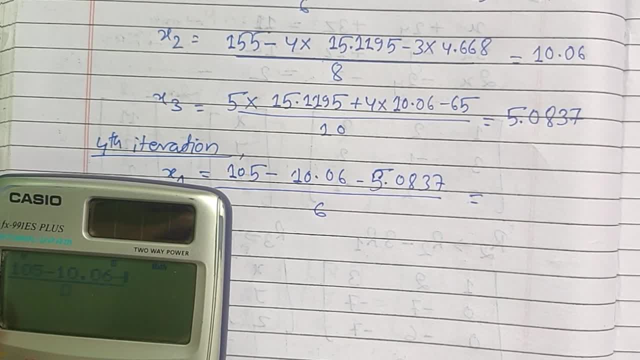 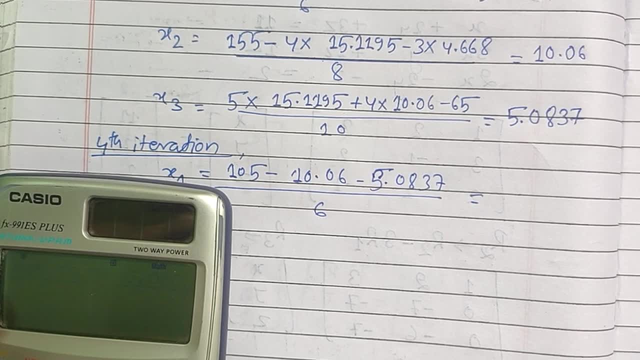 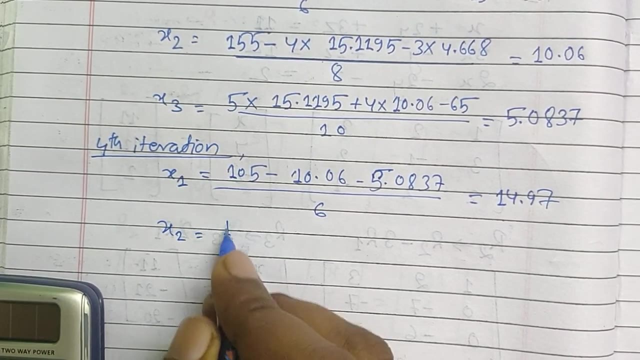 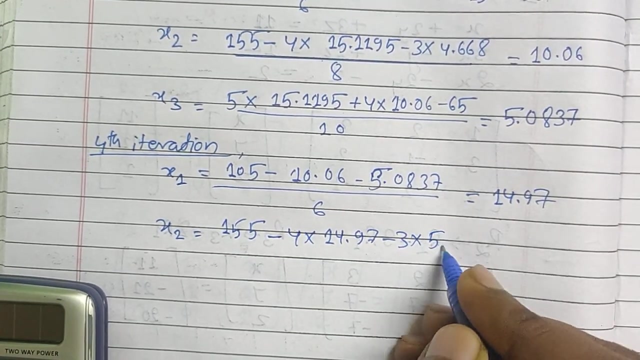 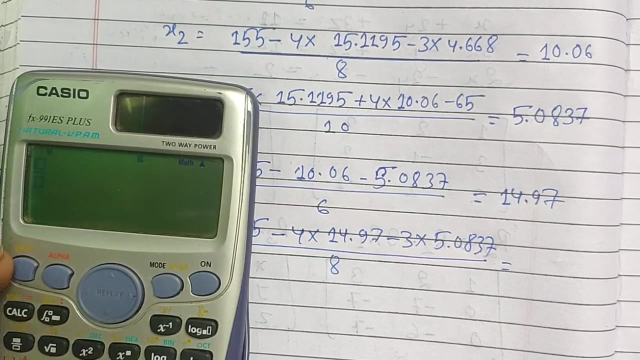 minus ten point zero, six minus five point zero, eight, three, seven divided by six, fourteen point nine, seven. similarly, x2 is equal to 155 minus four into fourteen point nine. seven minus three into x3 is five point zero, eight, three, seven divided by eight, which will be equal to one hundred fifty five minus four into fourteen. 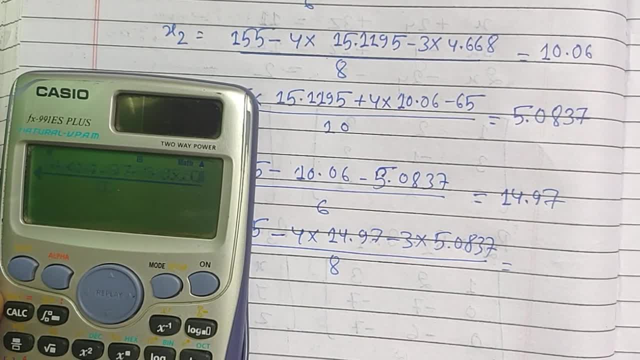 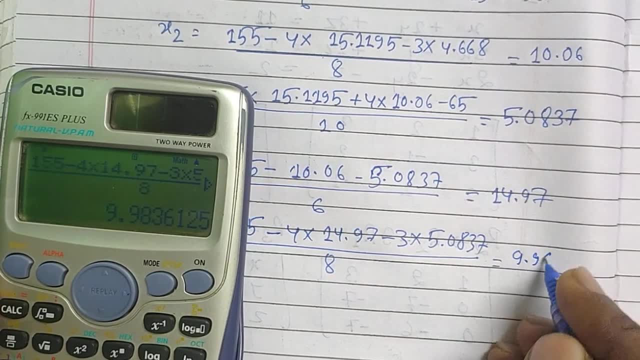 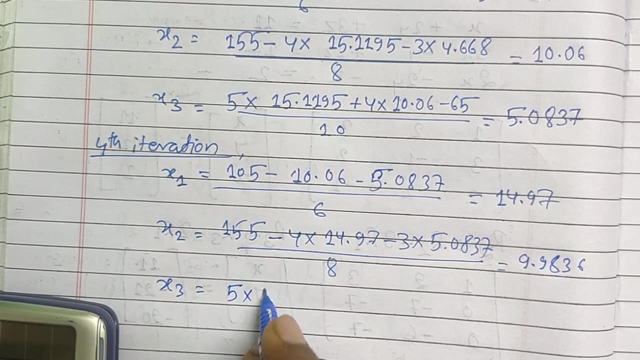 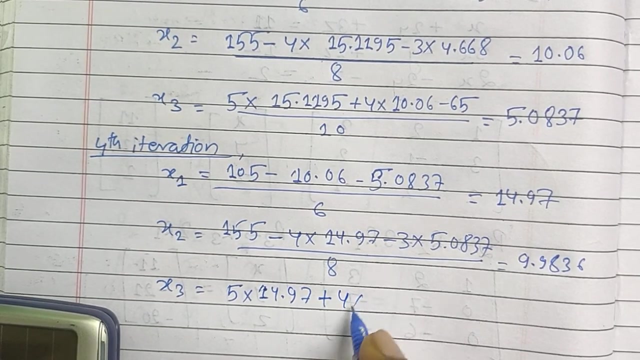 point nine, seven minus three into five. point zero: eight, eight, three, seven divided by eight, answer is nine point nine, eight, three, six. similarly, x3 is equal to five into five into action. fourteen point nine, seven plus four into x2. yanaki means nine point nine, eight, three, six minus. 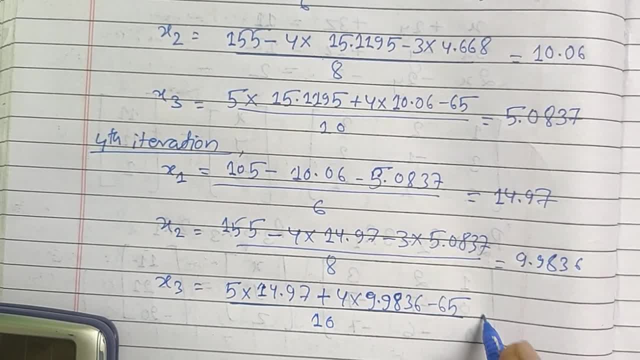 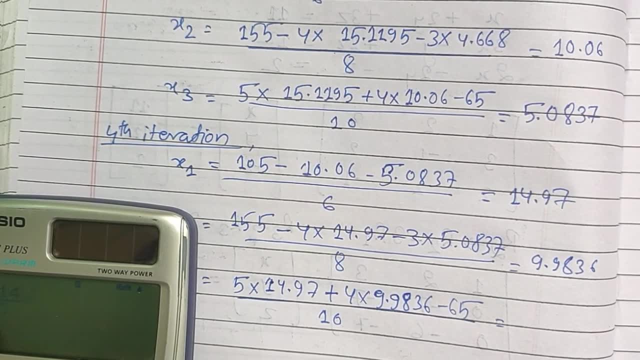 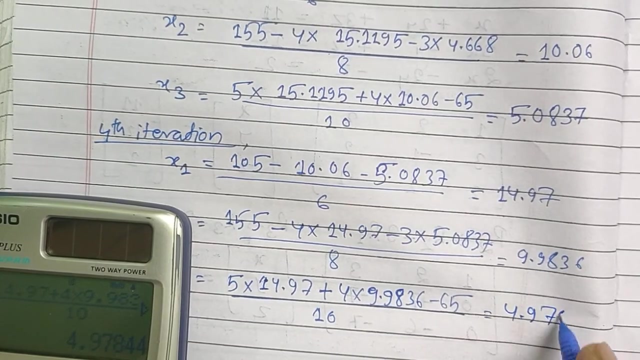 sixty five by 10. solve this. you will get 5 into 14.97, plus 4 into 9.9836, minus 65. divided by 10, answer is 4.97. eight four again. let's move toward the fifth. here i have calculated the value of the fifth. 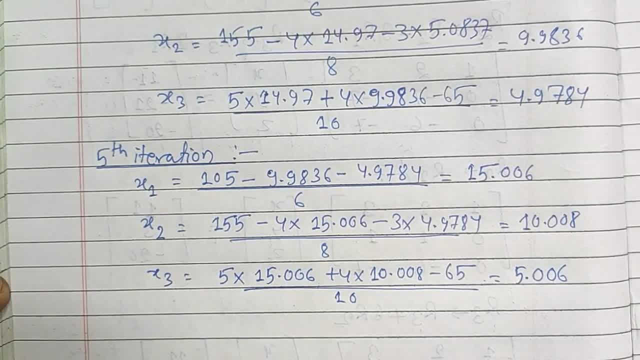 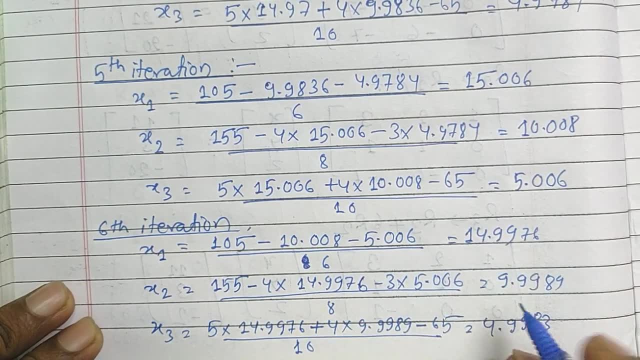 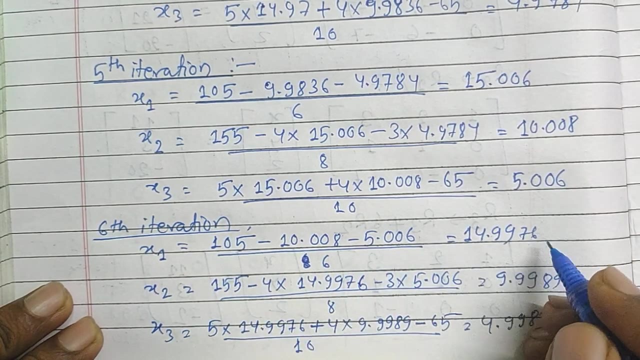 iteration. you can check it out by using the calculator. and let's move toward the sixth iteration. here, on finding the sixth iteration, we have got the value which is close to the value of the value of x1, x2, x3 in fifth iteration. so our x1 is x, approximately equal to 15.. x2 is